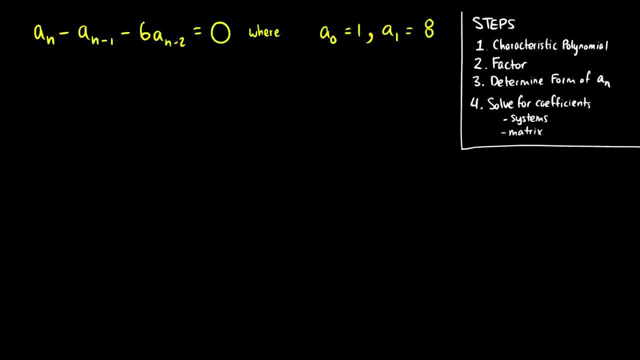 minus 1, minus 6, an minus 2 is equal to 0. It's a little bit challenging, so we're going to introduce an interesting concept here and I'm going to do this the very long way so we get each step. 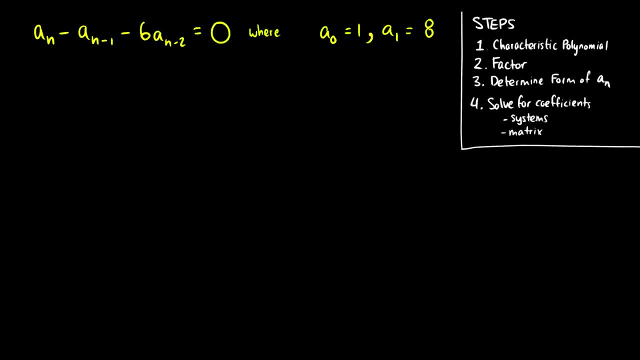 First of all, we want to transform this recurrence relation into an equation, So we need to get all of our an's to one side. Conveniently, this is already done. Now what we're going to do is we're going to multiply each term to the power, x to the n, and we raise it to the n because 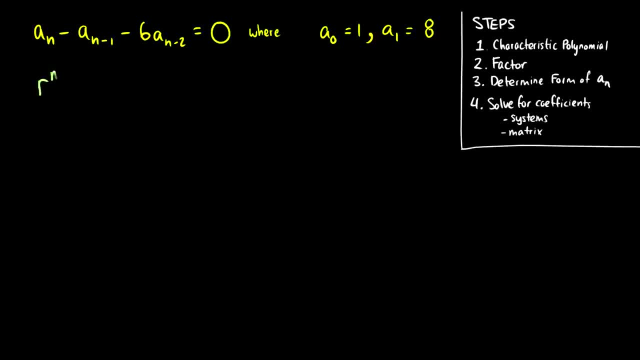 actually I should do this r to the n to be consistent with the other examples: r to the n, and this is consistent with the highest power here. So we have r to the n and we subtract r to the n minus 1, and we subtract 6r to the n minus 2.. 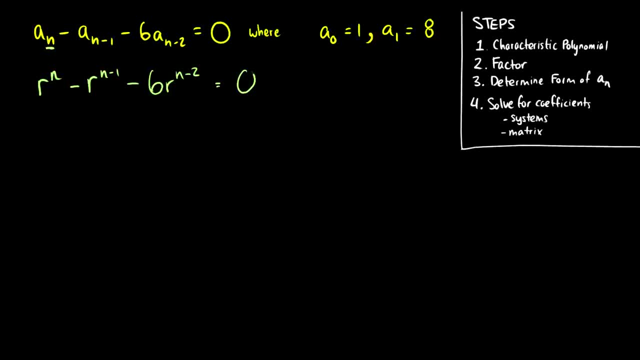 Okay, and this is going to be equal to 0.. So now we're going to divide by the lowest power of r here. so what we get is we're going to divide each term by r to the n minus 2,. 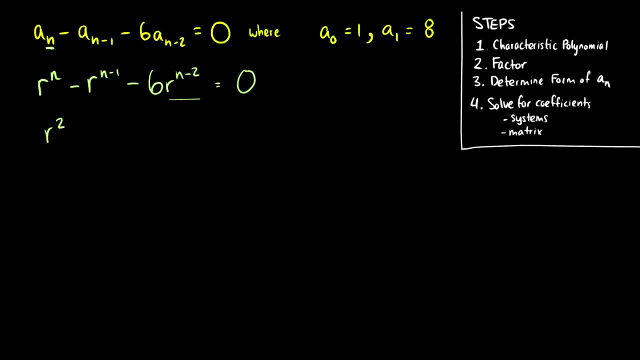 because it's the lowest one. So we're going to be left with r squared minus r. minus 6 is equal to 0. This was a complicated way of saying that. we take the smallest term and we just write it as a constant. we take the second smallest term, write it as a constant: times r. we take this the third. 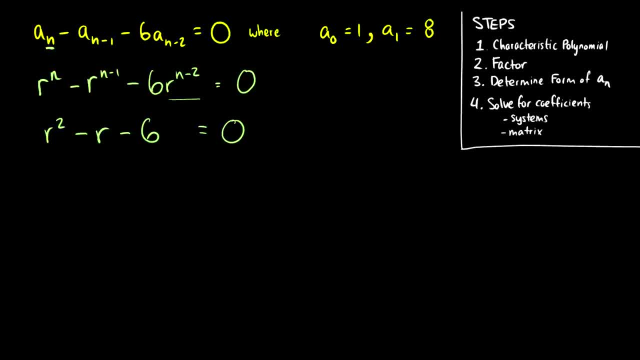 smallest term and write it as the constant times r squared, you can kind of see a pattern of how we got from this step to this step. So if the second step confused you don't worry about it. This is called the characteristic polynomial, So every recurrence relation has an equivalent characteristic. 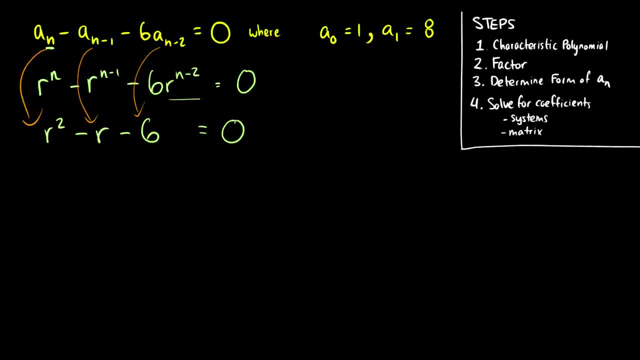 polynomial. This is step number one, So we want to get to this step. So, as an example, what if we had an minus 3 plus 2, an minus 2 minus 6, an minus 1 plus 7, an? What's the corresponding characteristic? 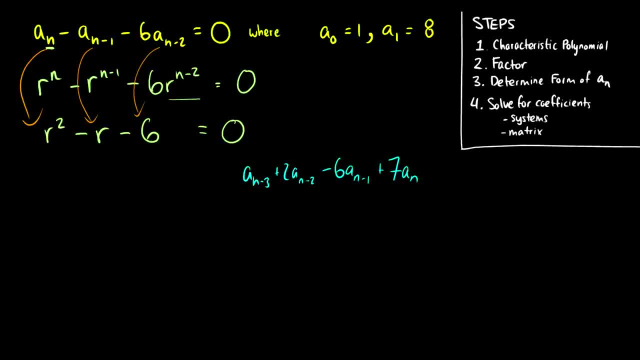 polynomial. Well, this: an minus 3 just becomes 1, because that's the coefficient. We have 1 an minus 3.. We get 2 an minus 2, the second smallest number. so this becomes plus 2r. an minus 1 becomes minus. 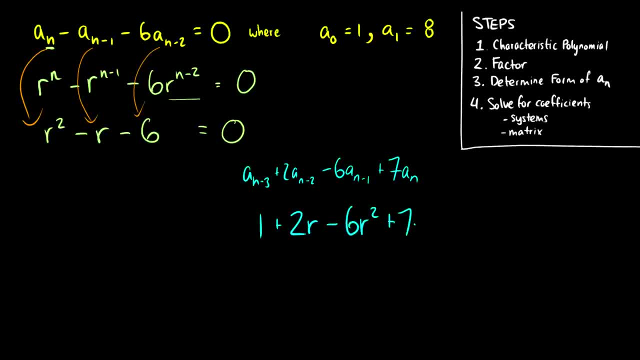 6r squared and 7r an becomes 7r cubed. so that is the corresponding characteristic polynomial. Okay, now the second step is to factor. So r squared minus r minus 6, what does this factor into? Well, this can be r. 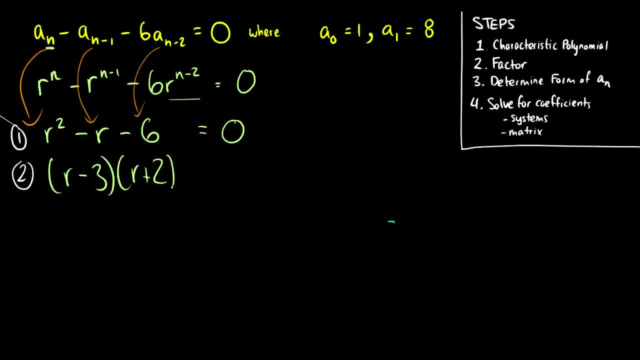 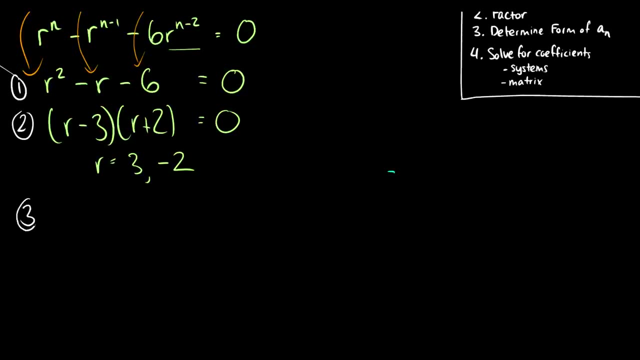 minus 3, r plus 2 is equal to 0.. So our roots are going to be: r is equal to 3 and r is equal to negative 2.. So what this means is that for step 3, the form of our solution, a, n, is going. 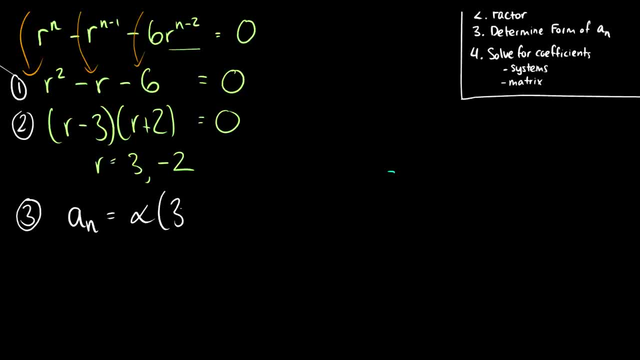 to be some number alpha times- 3 to the n- plus some number beta times negative- 2 to the n. The proof of why this works is a little bit long, but you can find it online in text form pretty easily. If I went over the form of why this works, this video would probably be at least 30 minutes. 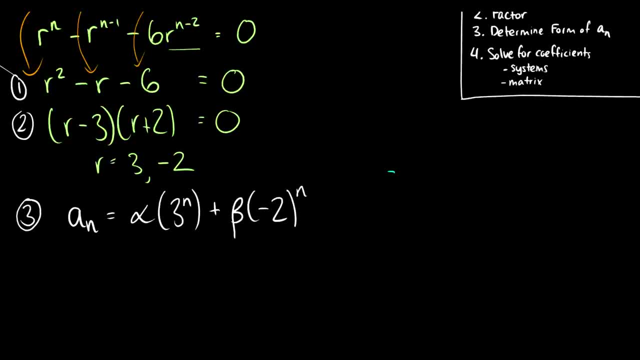 if I were to explain it in depth. So this is more of a mechanics guide rather than a theoretical guide. So, basically, our roots are going to be raised to some power n and we need some constants to modify that. So we're going to have some constants that are going to be raised to some. 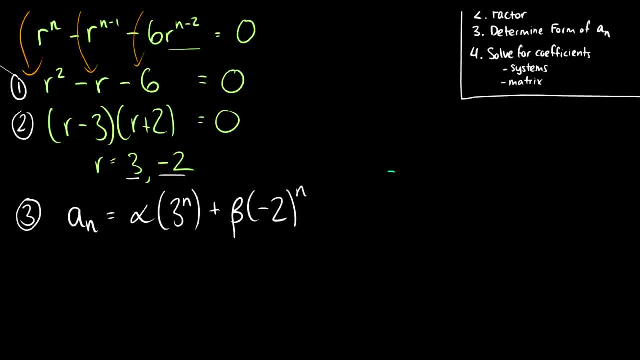 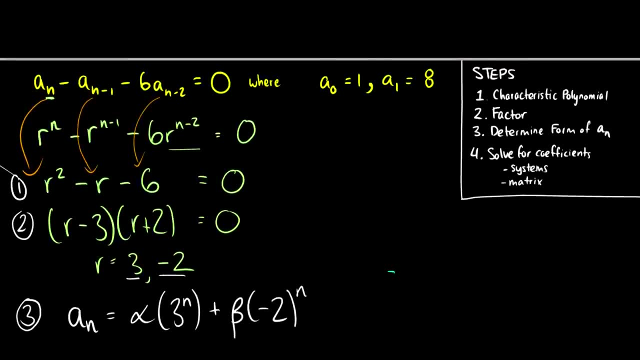 power n and we need some constants to modify that. So basically, our roots are going to be raised to some power n and we need some constants to modify that. So this is determining the form of a? n. Now we need to solve for some coefficients here. So what do we know? We know a 0 is equal to 1. 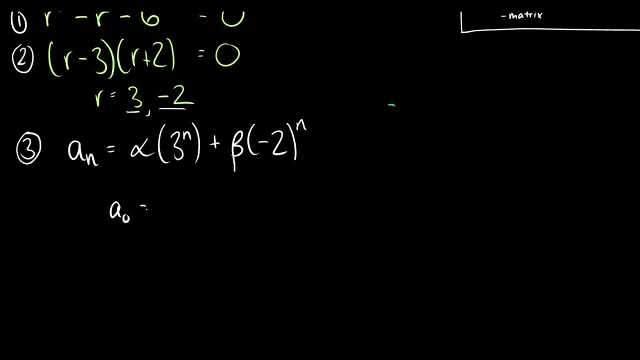 and a 1 is equal to 8.. So a 0 is equal to 1, a 1 is equal to 8.. So we have our form. so we need to solve for our coefficients. So let's plug some things in. Okay, so 1, we have a 0, so we take. 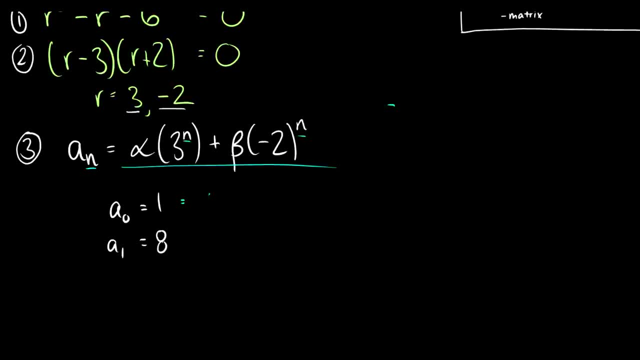 0 for our n's here. So alpha times 3 to the 0 is equal. sorry, 1 is equal to alpha times 3 to the 0, plus beta times. negative 2 to the 0 and 8 is equal to alpha times 3 to the 1, because we're dealing. 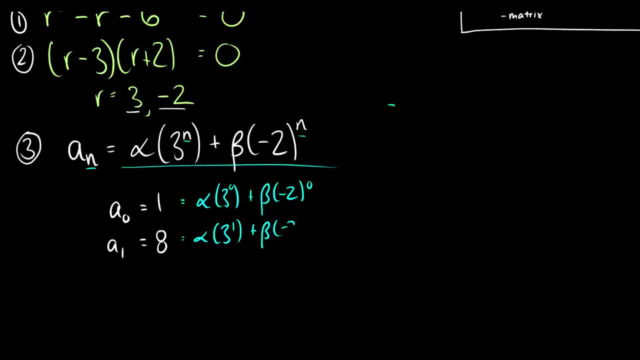 with a 1 plus beta times negative 2 to the 1.. So this is actually equal to a 1 plus beta times negative 2 to alpha plus beta, and a 1 is going to be 3 alpha minus 2 beta. Okay, so now we can. 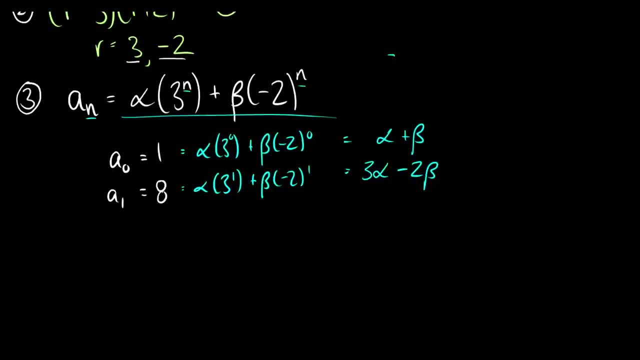 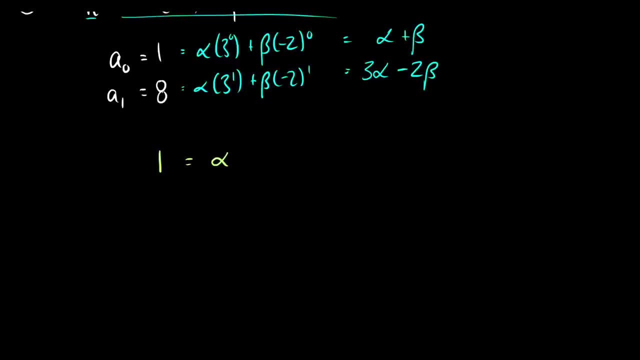 just add the equations up and see what we get. So I'm going to write this a little bit more compact here. 1 is equal to alpha plus beta. 8 is equal to 3 alpha minus 2 beta. Okay, so we want to add the first equation twice, so we'll do this step by step. So we multiply the. 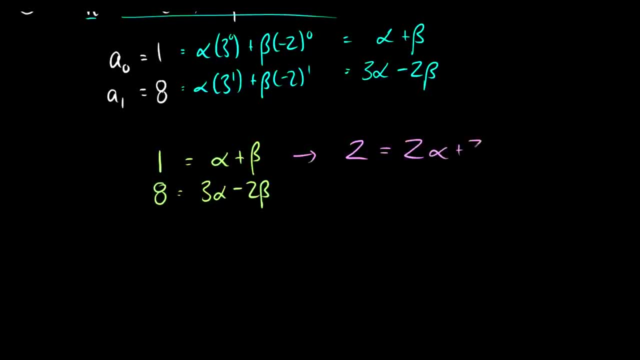 first equation by 2.. So 2 is equal to 2 alpha plus 2 beta. We keep the second equation the same: 8 is equal to 8.. 8 is equal to 3 alpha minus 2 beta. and now we can add these up to solve for alpha, So 10,. 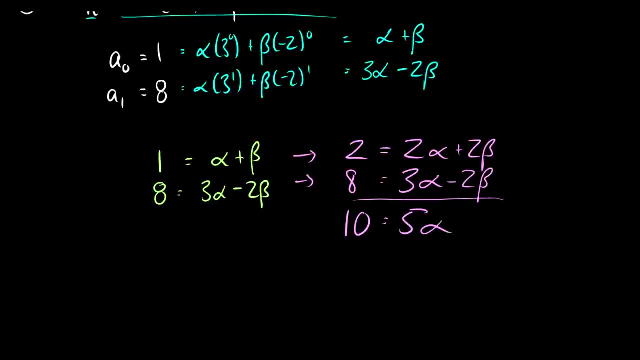 is going to be equal to 5 alpha, because 2 beta minus 2 beta it cancels. So now we know that alpha is equal to 2.. OK, so using this equation we have: 1 is equal to 2 plus beta. 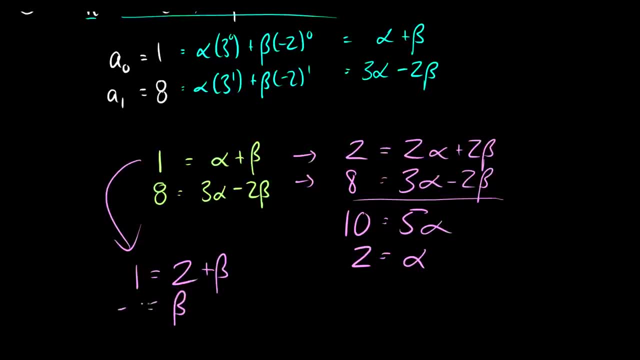 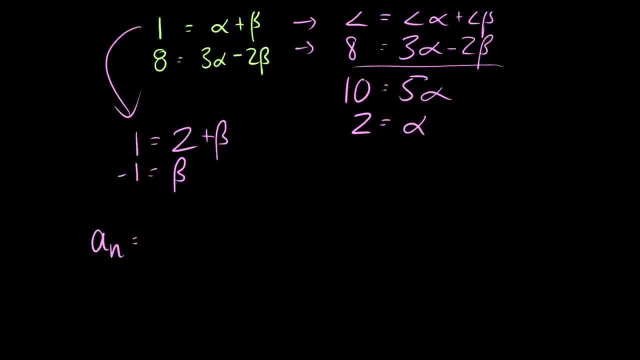 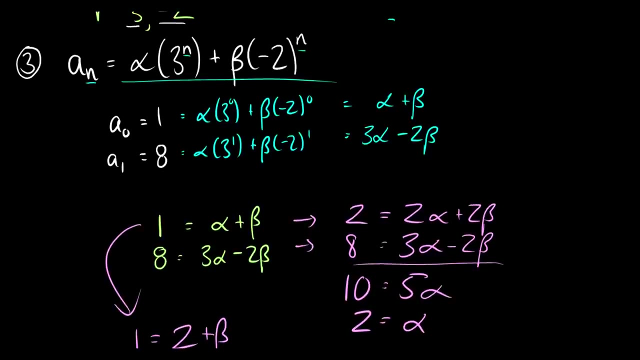 So beta is equal to negative 1.. OK, now an when we plug in our alpha and beta values. in fact I'll just do this back up in the original part here: alpha is equal to 2 and beta is equal to negative 1.. 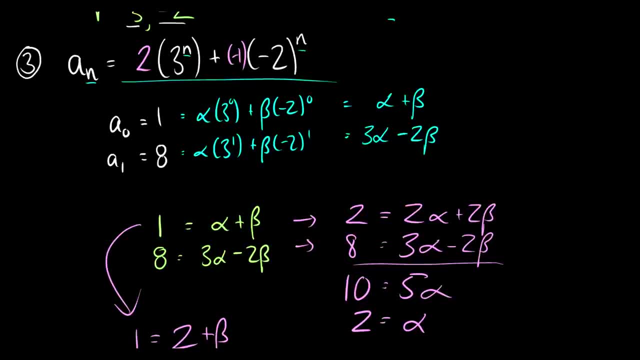 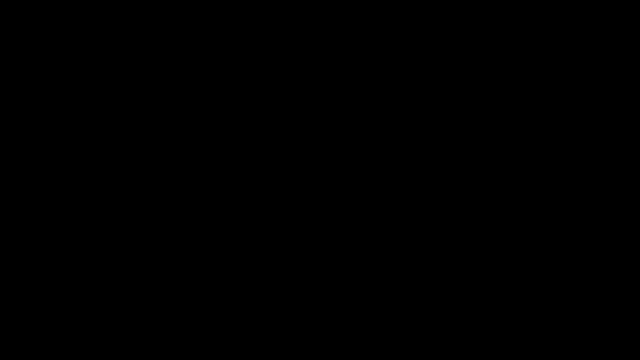 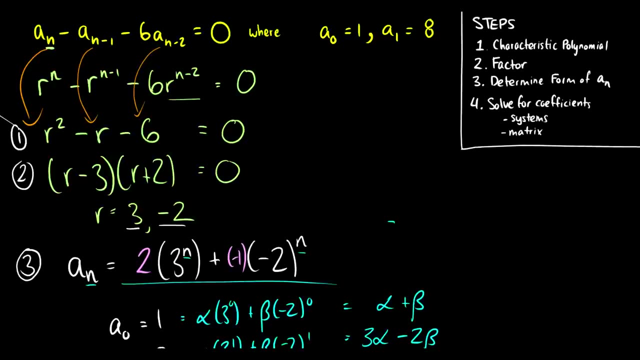 So that is the solution to our homogeneous equation. So we can test it out, We can make sure it works. OK, that's a little bit too far. How should I do this, OK? well, we have some rules. We have some room over here. 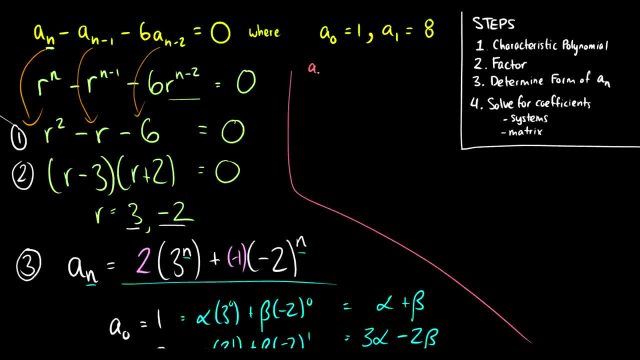 So we'll use this room. a0 is equal to 1.. a1 is equal to 8.. So how do we find a2?? OK, well, a2, we have to put some things on the other side. So, more generally, we know that an is equal to an minus 1. 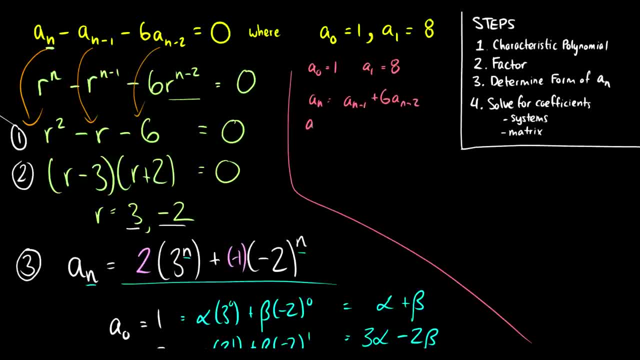 plus 6, an minus 2.. So a2.. So a2.. a2.. So a2.. a2.. 6a1, sorry, just a1 plus 6a0.. So this is going to be 8 plus 6 times 1, which is 14.. So a2 is 14.. 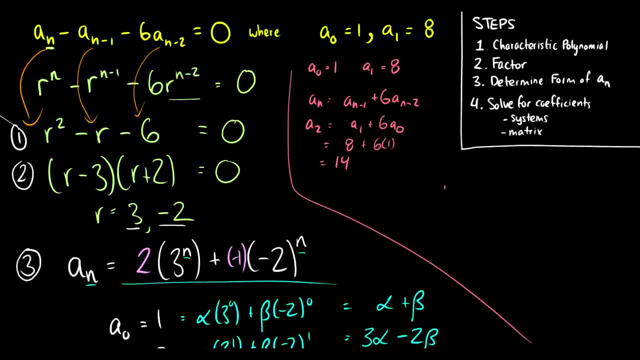 Let's see if our formula gets the same answer. a2 will be 2 times 3 squared, plus negative, 1 times negative 2 squared. So this is going to be 2 times 9 minus 4, which is 18 minus 4,. 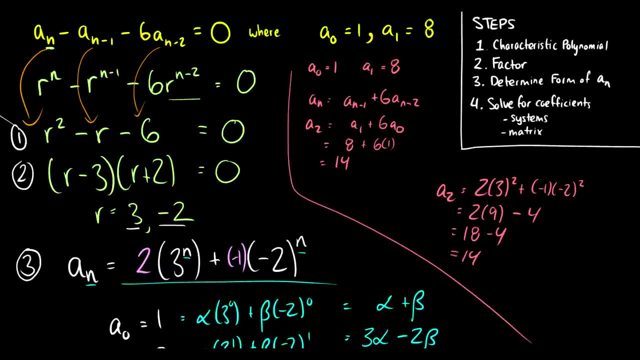 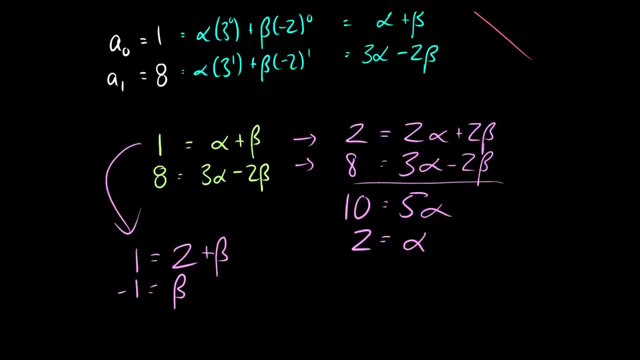 which is equal to 14.. So our formula gets the same result that our recurrence relation does. Again, this can be difficult. This is a long and challenging problem, So go through each step very, very carefully and go through solving for your coefficients carefully. 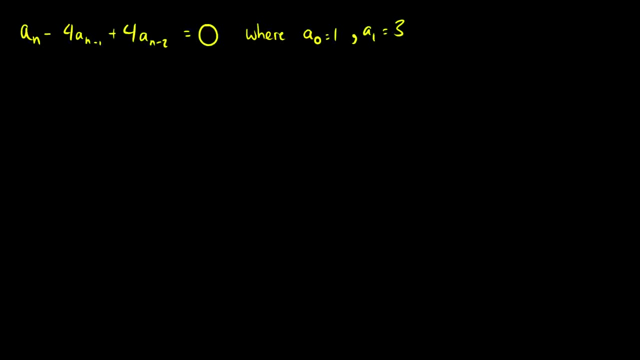 That was one example, So of course we'll do another example: an minus 4an minus 1, plus 4an minus 2 is equal to 0.. a0 is equal to 1.. a1 is equal to 3.. Let's get the characteristic polynomial. 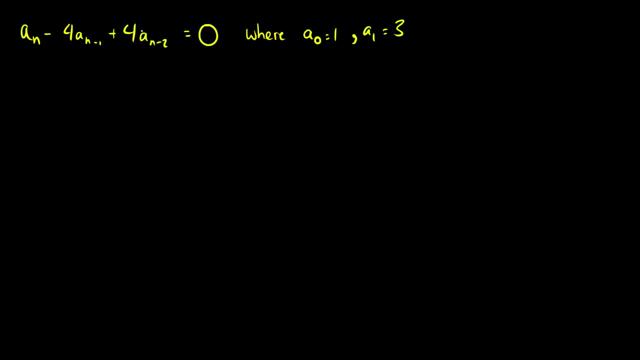 So an minus 4an minus 1 plus 4an minus 2 is going to have the characteristic polynomial r squared minus 4r plus 4. is equal to 0.. Okay, so this is going to be r minus 2 times r minus 2 when we factor it. 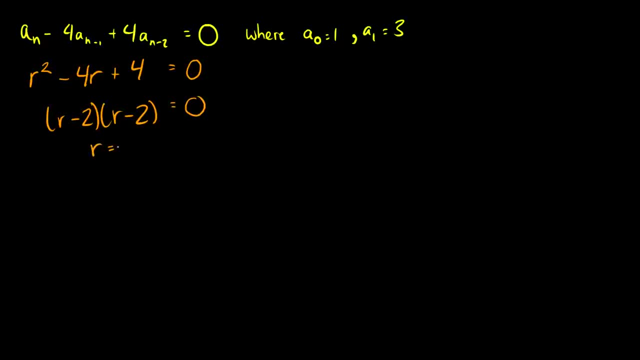 This is equal to 0. So our roots are 2 and 2.. So this means that our formula an should be some number alpha times 2 to the n plus some number beta times 2 to the n. Then shouldn't alpha and beta be the same number. So we get a weird situation here. 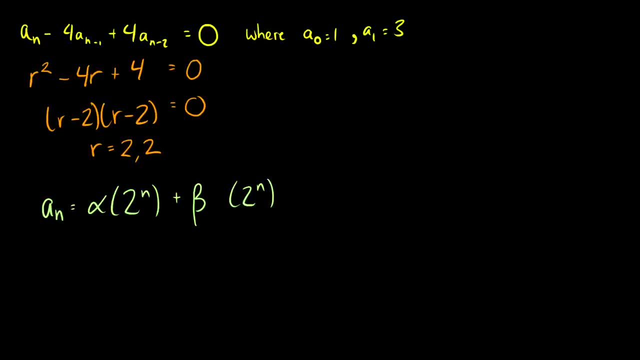 So normally I'd say this is okay. But what happens when we have similar roots is say we have 2 to the n, then our second one is going to be n times 2 to the n. Suppose we had another root of 2.. Then our 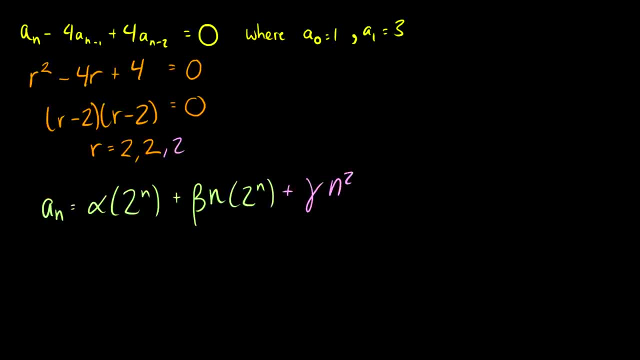 third one would be gamma n squared times 2 to the n. We'd have to multiply by n squared to have another root of root, 2.. Another root of 2.. So when we do forms, if we ever have similar roots, then we 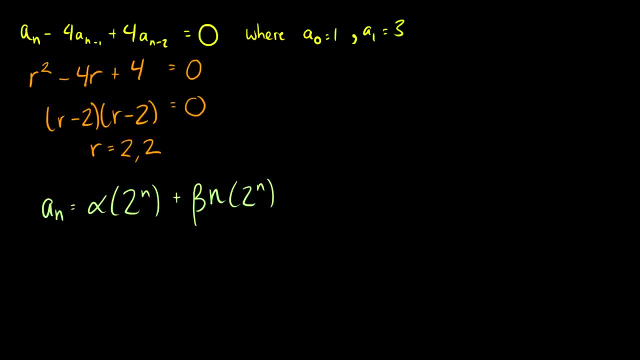 simply just multiply by n however many times you have it in there. So we already have 2 to the n once. So we multiply 2 to the n times n. Okay, Let's do what we did before. A0 is equal to 1, which when we plug in 0 in the ns here, we just get alpha. 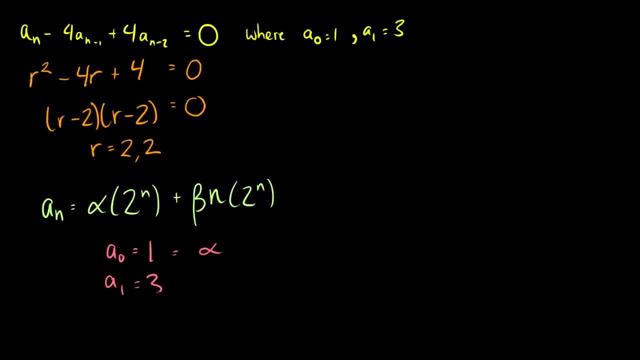 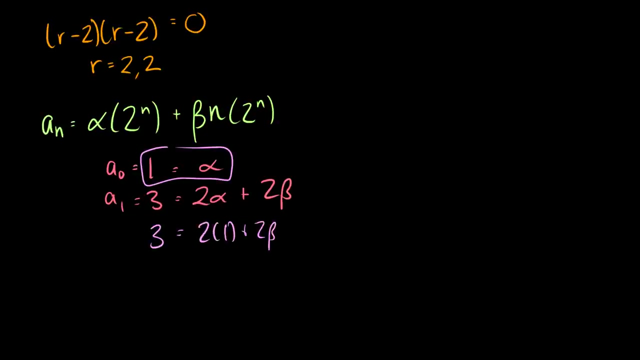 A1 is equal to 3.. So this will be 2 alpha plus beta times 1 times 2 is 2 beta. So fortunately we already know that alpha is equal to 1.. So b1 is equal to 3.. So g is equal to 1.. So 4 to the n times 1 plus 2 beta. So 3 is equal to 2 times 1 plus 2 beta. So 1 is equal to 2 beta. So 1 half is equal to beta. 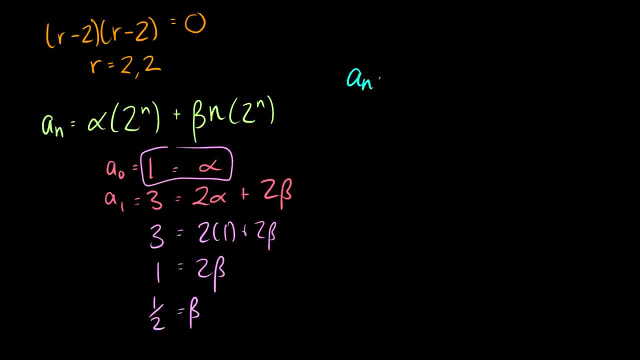 So when we solve our recurrence relation here we get: An is equal to 2 to the n, because alpha is equal to 1, plus 1 half n, 2 to the n. Let's do that again, Okay, Okay. 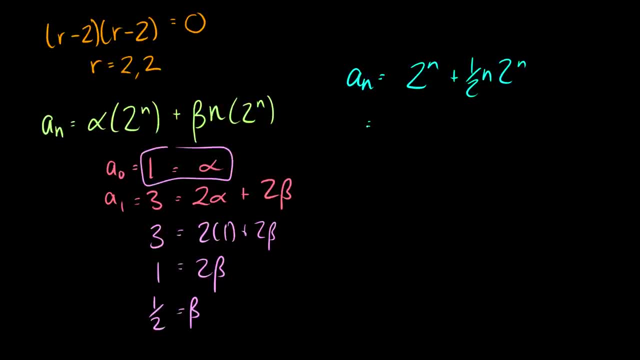 Okay, Okay to the n. So let's actually factor out a 2 to the n here. So this is 2 to the n times 2 to the n times 1 plus 1 half n. Okay, that would be our solution here. In fact, we could actually simplify. 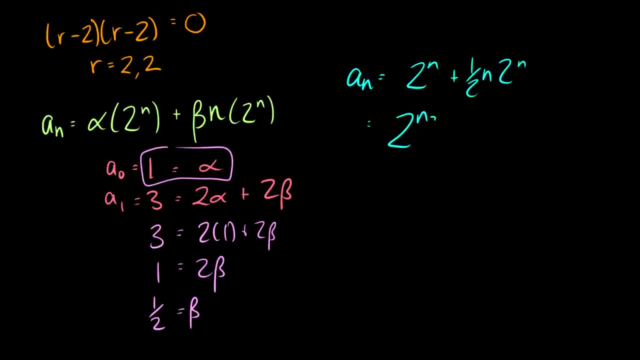 this a little bit nicer. We could factor out 2 to the n minus 1.. Actually I should do one step. first, 2 to the n plus n times 2 to the n minus 1, because we just divide 2 to the n by 2.. And then 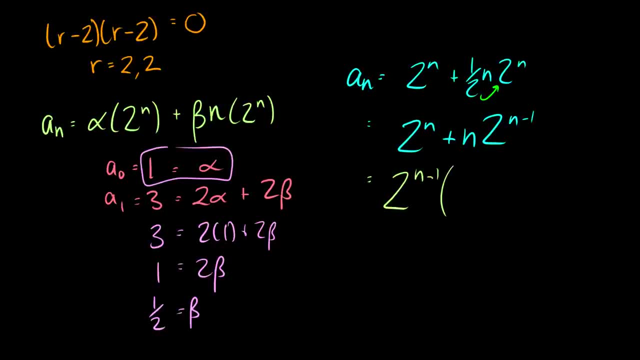 we could pull out a 2 to the n minus 1 and this is just times 2 plus n. So that's another way we could do it And that is the solution to the recurrence relation And you can plug in some numbers yourself and see if you can solve them. So this is homogeneous recurrence relations. 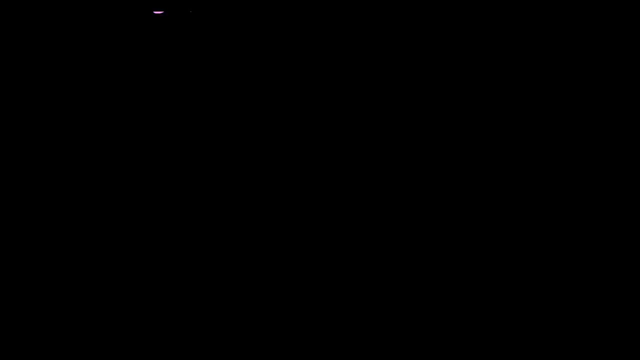 The most important part is the characteristic polynomial. So if you have roots that are different, then your a? n. So okay, let's say that r is equal to all the numbers And you have all these different roots and they go up to some number, n. then our solution is going to be of: 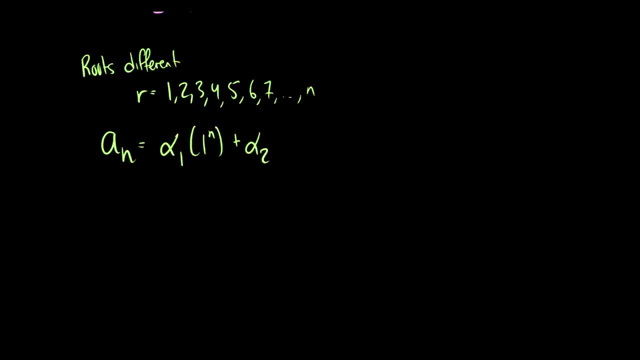 n times 1 to the n, plus alpha 2 times 2 to the n, plus alpha 3 times 3 to the n, all the way up to some number: alpha n times n to the n. I probably shouldn't have picked n for this, So I'm going to. 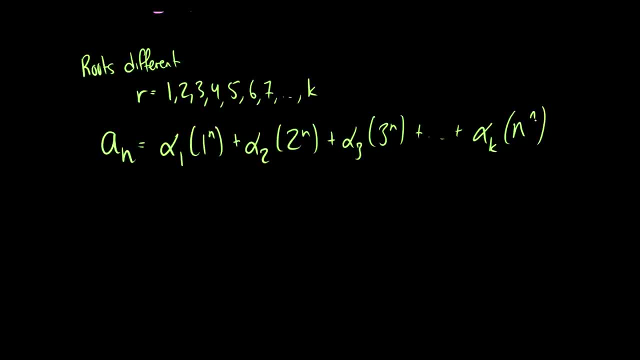 pick k, It goes all the way up to number k. Okay, that's a little bit nicer. Okay, so that's when the roots are different. This is going to be the form of your answer. then you're going to have to solve a hell of a lot of equations to get your result. Now, when you have roots, the 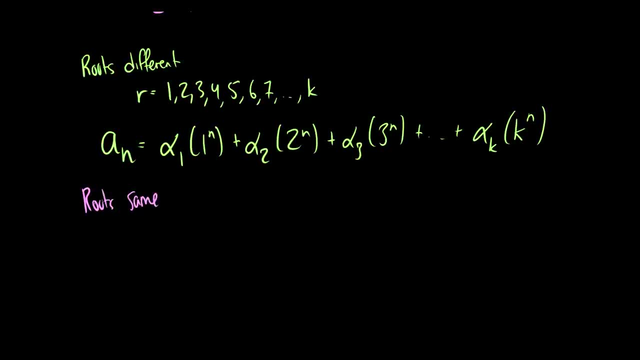 same. So let's say r is equal to 1,, 1, 1.. No, let's not do 1.. Let's do 3,, 3,, 3. And we do 3k times And then we get a bunch of 2s. 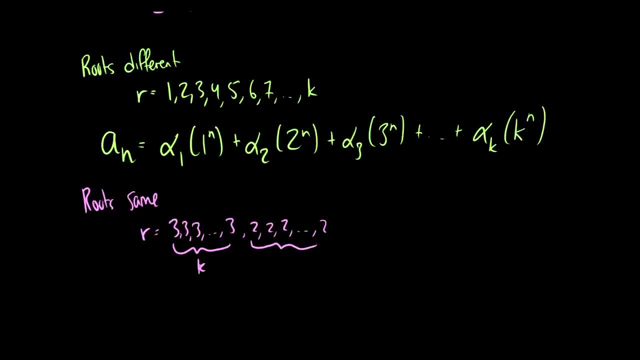 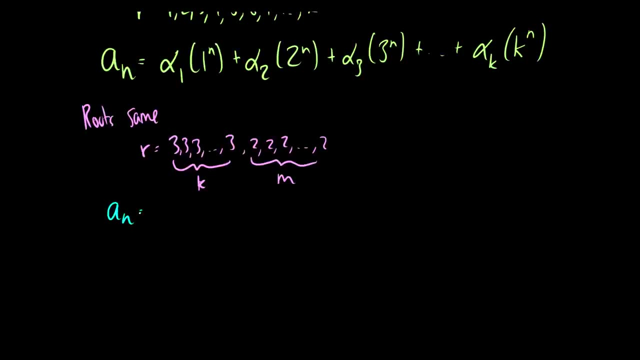 And we'll say this is 2,, this is m times. then our form a n is going to be alpha 1 times 3 to the n, plus alpha 2 n times 3 to the n, plus alpha 3 n squared times 3 to the n, And this will add all. 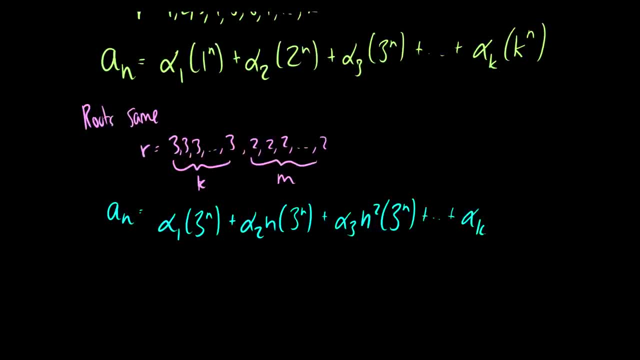 the way up to alpha 2, n times 3 to the n. And then we're going to have to solve a hell of a lot of equations to get the answer. So let's say r is equal to alpha k, n to the k times 3 to the n. So 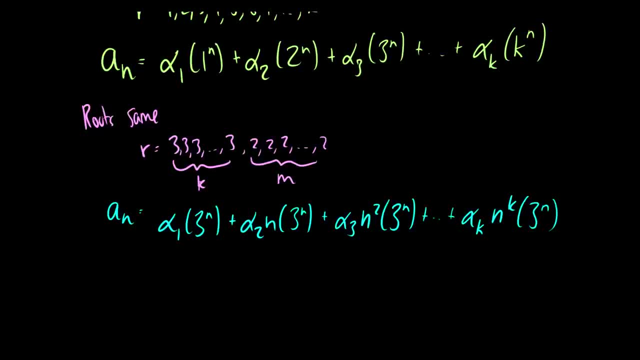 this is 3 to the n k times. So our final time we added up should be alpha k times n to the k times, 3 to the n, And then we add up, of course, our 2s. So we have beta 1, 2 to the n plus. 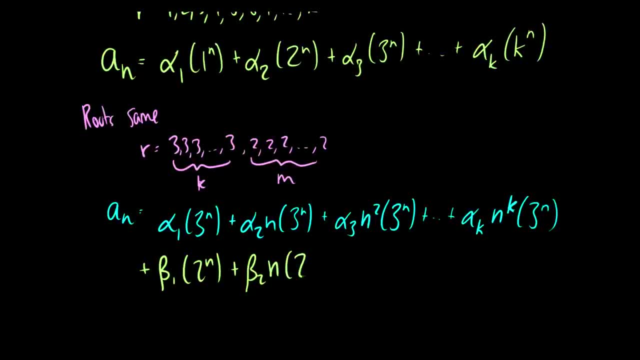 beta2 times n, 2 to the n, and then we add all the way up to beta, so it's beta m times n to the m, 2 to the n. So a little bit of heavy notation but I hope you get the concept that you. 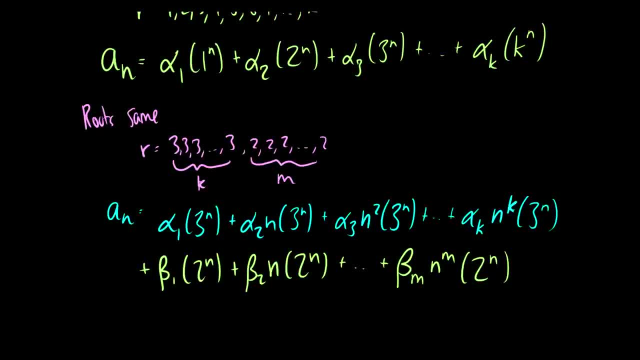 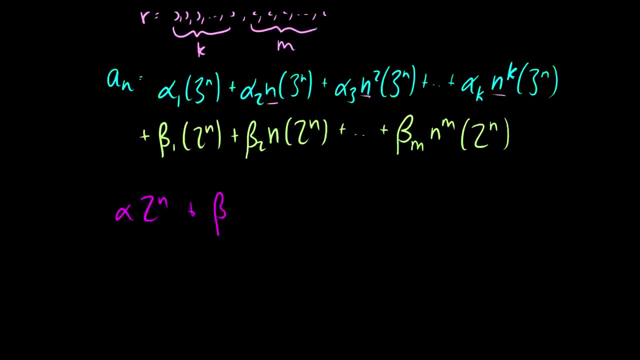 have to multiply. you know the amount of roots you have by your numbers n here. So that way let's say we have, for instance, let's have, alpha 2 to the n plus beta 2 to the n. If we have this, 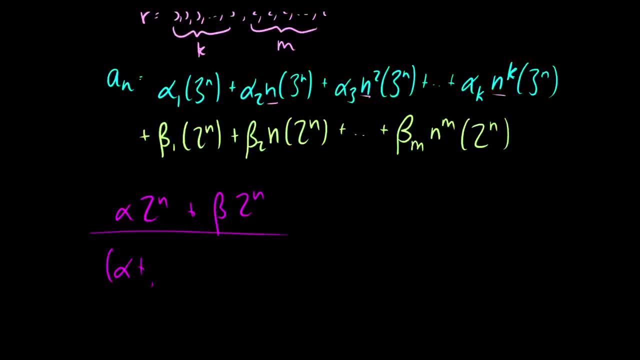 result. really, it's the same thing as saying alpha plus beta 2 to the n, but we know this can't happen because if this did, then it would be geometric, But it's not geometric. so we clearly need something else in here to prevent it from. 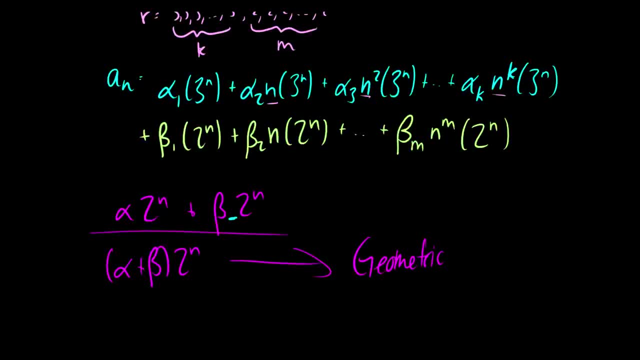 being geometric, So this is why that doesn't work. All right. so those were the two examples I'm going to do, and the last one is word problems. I'm not going to solve this, but I'm going to show you how. 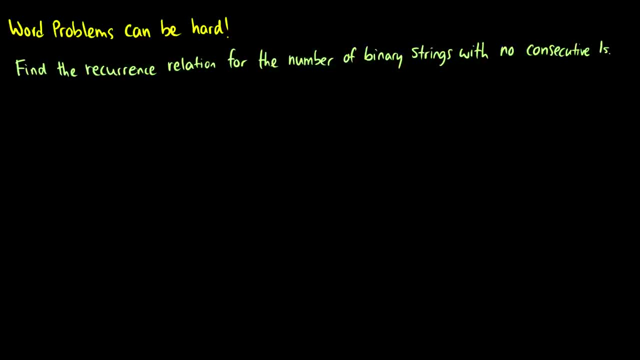 to take a word problem and turn it into a recurrence relation. So let's find the recurrence relation, So the number of binary strings with no consecutive ones. Okay, so let's be a little bit tricky here. We're going to take the nth number, so a to the n is the nth number and this is going to be equal. 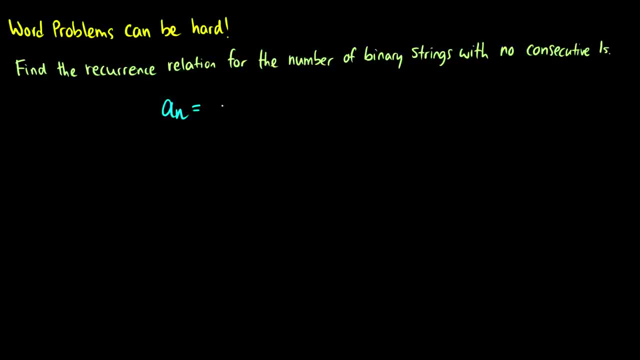 to all of the strings of length n that end in a zero, plus all of the strings of length n that end in a 1.. So if we have a bunch of numbers and this is the nth digit, then it can be either a zero or a 1.. 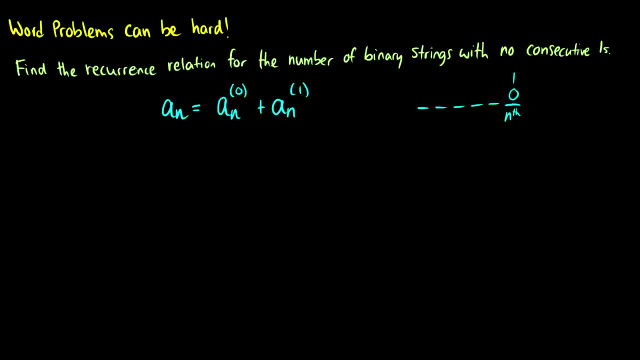 So we're going to separate the two. If the digit ends in a zero, then we can have any number prior, so the rest can be taken as is. If the word Ends in a number prior, then we have any number before this And then in the. 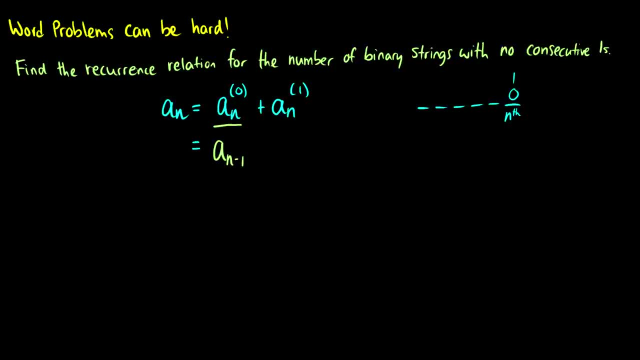 a n minus 1 ways. However, if the last digit is a 1,, then we can write the rest in a n minus 1 ways, but the n minus 1, so let's say this is 1,, because we can't have any consecutive 1s. 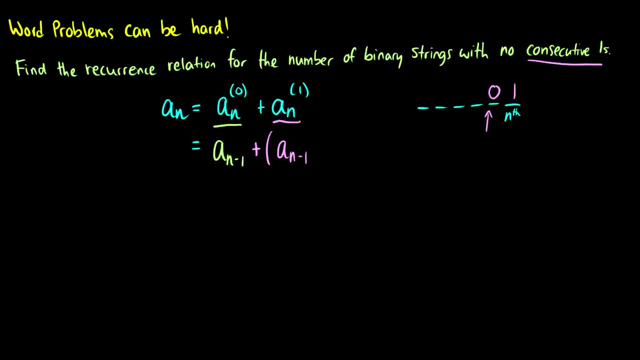 this number right here has to be a 0. So it can only be the fact that a n minus 1 has to end with a 0. Okay, which means that a n minus 1 plus well, if a n minus 1 ends with a 0,. 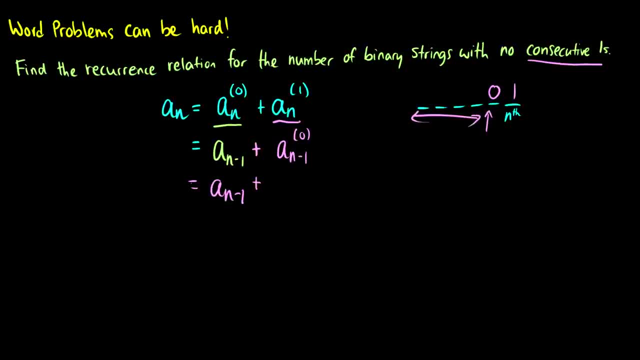 then the rest of the sequence. a n minus 2 can be anything they want. So a n minus 1 plus a n minus 2, and this is the recurrence relation. Of course we need to know that. how many ways can we have 0, or a string of length 0, 1? How many ways can we have a string? 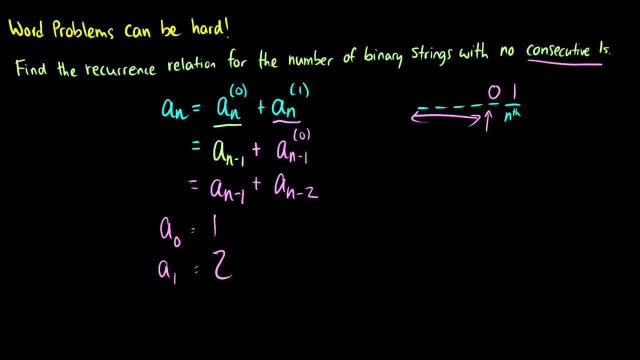 of length 0, 1?. How many ways can we have a string of length 0, 1?? How many ways can we have a string of length 1?? It can be either 0 or 1, so it would be 2.. And this is your recurrence relation. So. 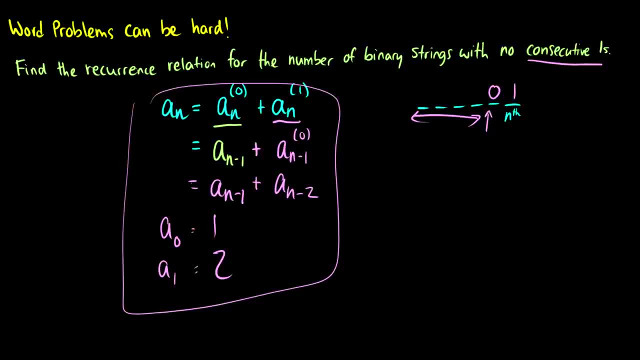 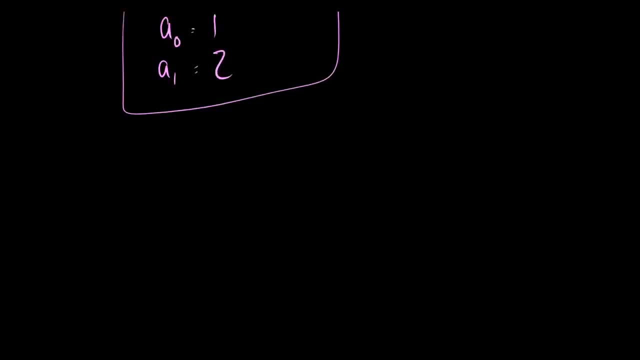 the number of binary strings with no consecutive 1s can be found with this recurrence relation And again to sort of go over the example and why I did it a certain way, suppose we have a binary string of length n. this is some n. It can either end with 0 or 1,. so we say 0 or 1.. And again, to sort of go over the example and why I did it a certain way, suppose we have a binary string of length n, this is some n. It can either end with 0 or 1,. so we say 0 or 1.. And again, to sort of go over the example and why I did it a certain way, suppose we have a binary string of length n, this is some n. It can either end with 0 or 1,. so we say 0 or 1.. And again, to sort of go over the example and why I did it a certain way, suppose we have a binary string of length n, this is some n. It can either end with 0 or 1,. so we say 0 or 1.. And again, to sort of go over the example and why I did it a certain way, suppose we have a binary string of length n, this is some n. It can either end with 0 or 1,. 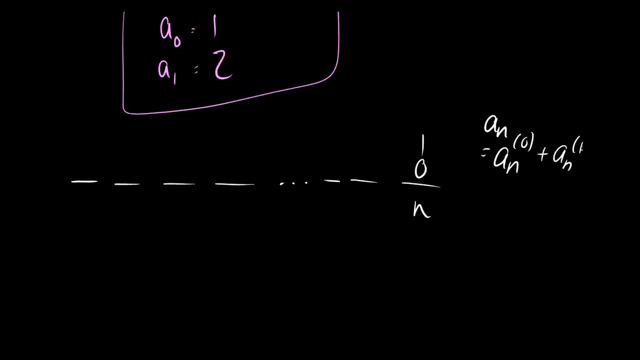 so we say 0 or 1.. And again, to sort of go over the example and why I did it a certain way, ends in 0 plus a n that ends in 1. the number in brackets above it are ends with. so the number of ways that the recurrence relation can end is with 0 or 1. so if it is a 0, 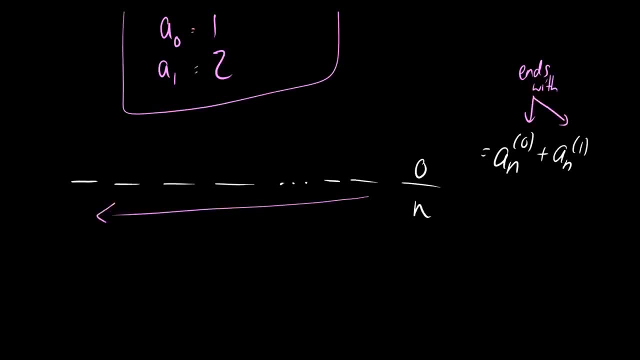 then all of these ways can be written however they want. so that's going to be a n minus 1, because there's a n minus 1 ways to order the rest. if, however, n ends with a 1, then this n minus 1 has to be a 0, so then the rest can be ordered in a n minus 2 ways. so there's two cases we have. 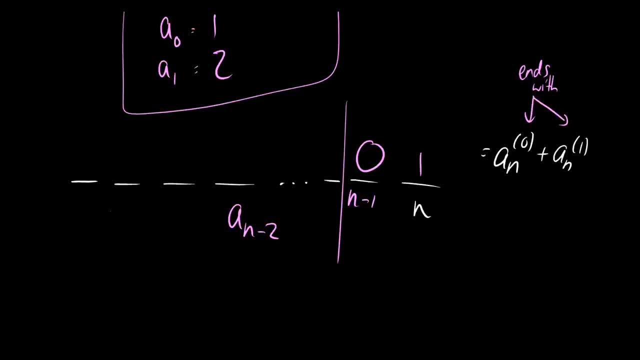 to deal with. so that's just the thought process of how we go through this thing. so in the end we get a n is equal to a n minus 1 plus plus a n minus 2.. Where does this seem familiar? Where does this seem familiar? I swear we've seen this before. 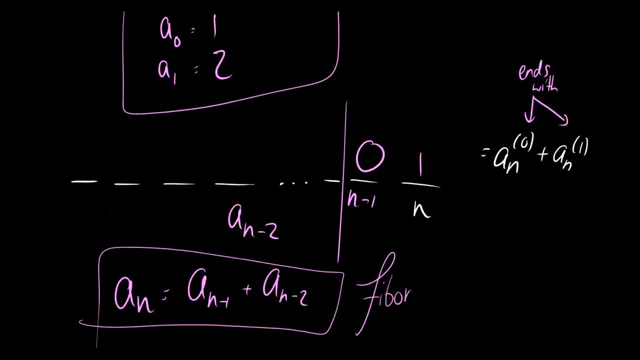 In fact we have. this is Fibonacci. So what's this doing here? It's kind of weird Just being up in binary strings. Well, they're actually related. Fibonacci is a very, very common sequence seen in a lot of relations that you 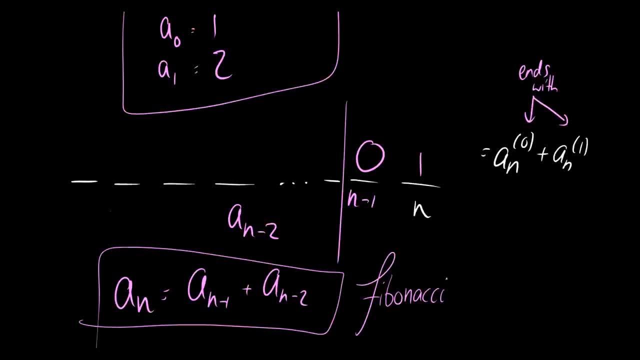 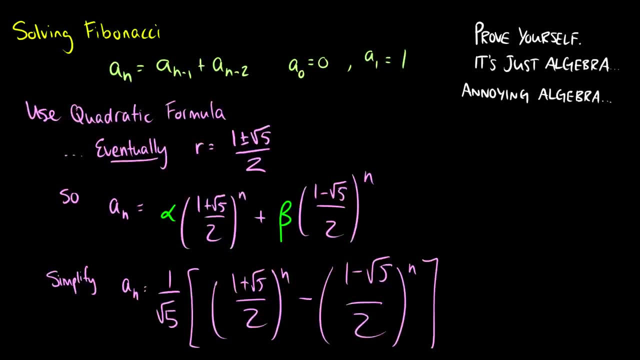 wouldn't expect. So it's probably best if we solve for it, right, If we know what Fibonacci looks like as a formula, And I could solve the whole thing on camera. but I'm bound to make a mistake. And I'm bound to make a mistake because the algebra 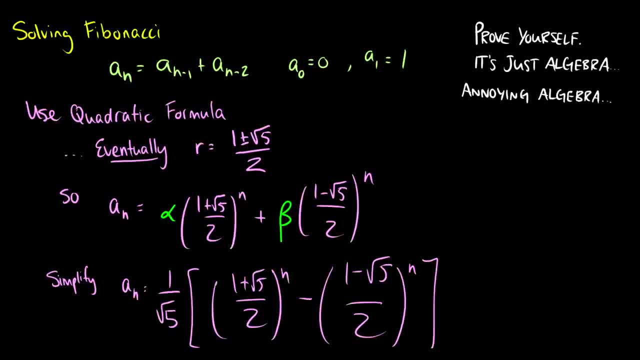 is very difficult, and talking while writing and doing math is not the simplest thing to do, So instead, I'm going to give you a skeleton of what's going on. So a n is equal to a n minus 1 plus a n minus 2.. 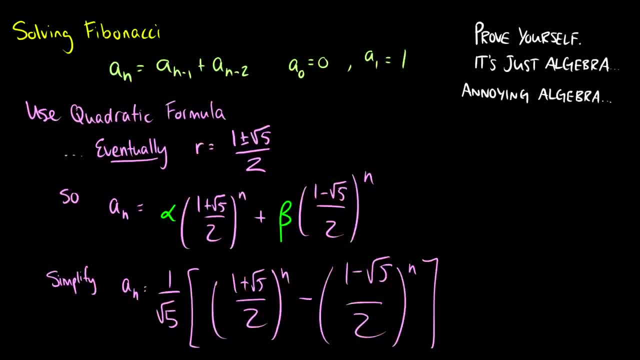 Our first two numbers are 0 and 1.. So what we do is we have to find the characteristic polynomial. So we get a n minus a n minus 1, minus a n minus 2 is equal to 0. So we get r squared minus r minus 1 is equal to 0.. 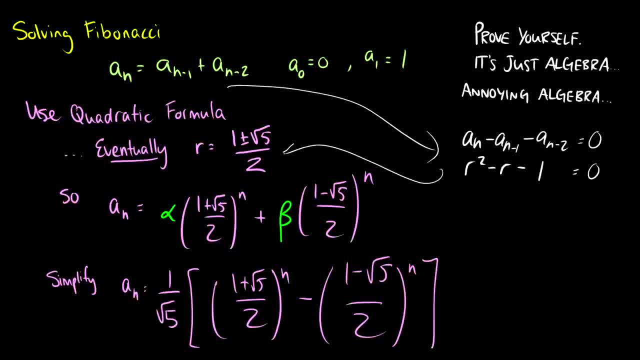 Using the quadratic formula, we get that r is equal to 1 plus 1.. Plus root 5 over 2 and 1 minus root 5 over 2.. So then we get this form: alpha times: 1 plus root 5 over 2. 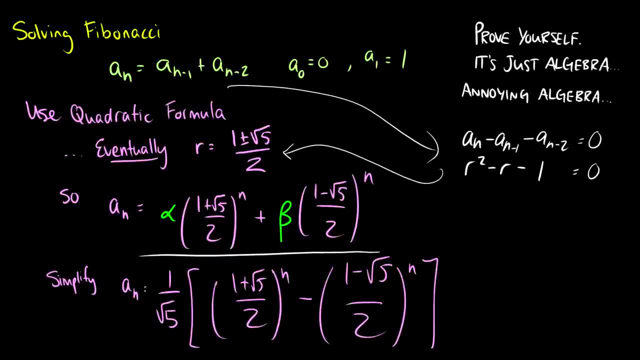 to the n plus beta times 1, minus root 5 over 2 to the n. And then when we solve for our coefficients a0 and a1, we end up getting that a n is equal to 1 over root 5 times 1. 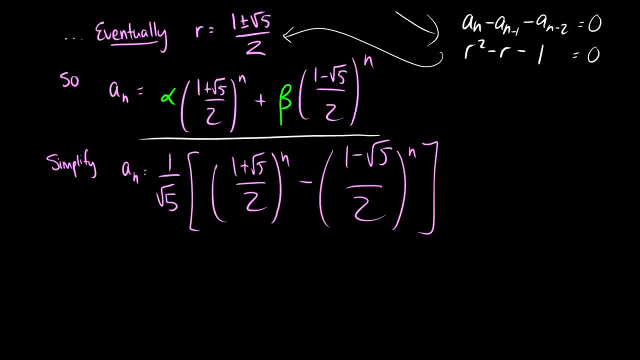 plus root 5 over 2 to the n. minus 1. minus root 5 over 2 to the n. All this is is algebra. This technique follows the exact same method that we did for the previous question And, as your homework, I challenge you to do the algebra and get this result to prove that. 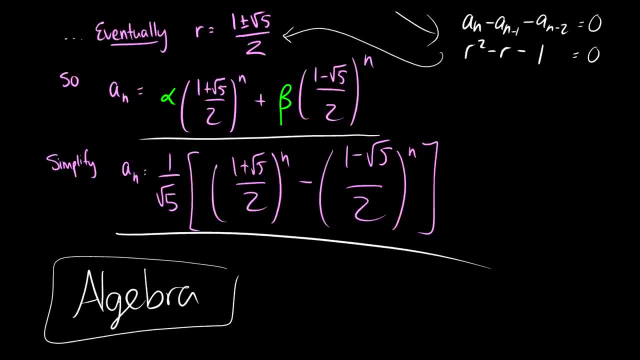 you can do it. If you have any questions on how to do this, leave it in the comments below and I will answer them, Because if you can do this, if you can solve this with the skeleton and understand why each step works, you understand homogeneous recurrence relations and how to. 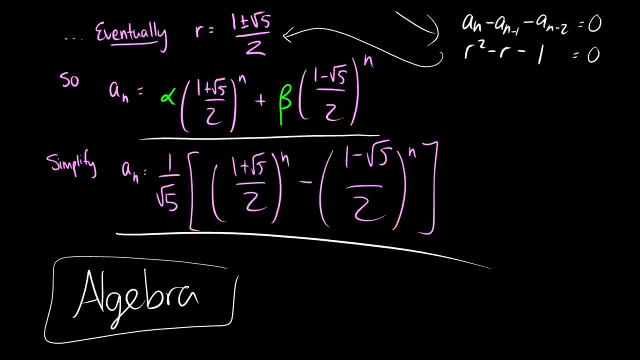 solve them. So that is your goal: Do this. and if you can't get this, leave them in the comments below and I will explain step by step how to do this, But I want to avoid this for now. There is also some more practice questions on the midterm at trovetutorcom in the Discrete.